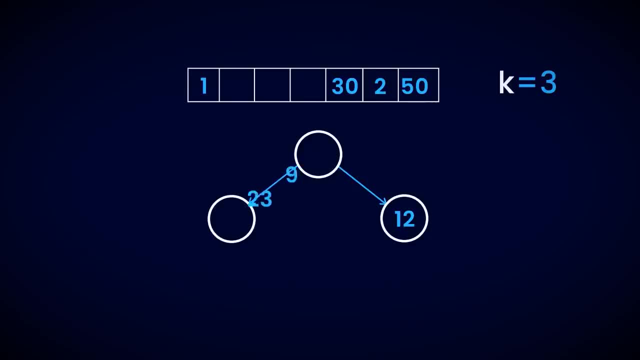 we add it to the heap and right after doing that we remove the minimum number from the heap. This way we maintain the heap size of K and the heap always contains the largest K numbers. we have seen so far This step of adding and removing the number to the heap. 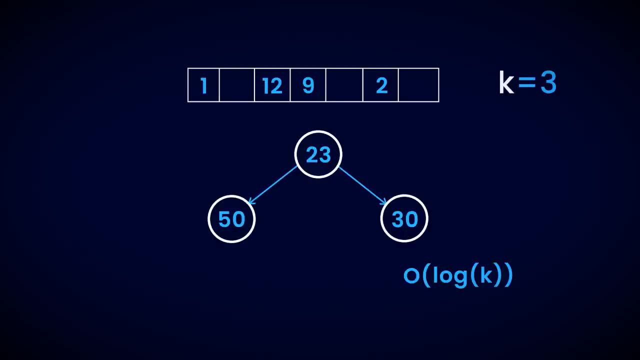 has a big O of log K and we do this for every number in the array which is n times. So the big O of the Top K Elements Algorithm is n log K, which is better than n log n, which we got through sorting. At number 4, we have the sliding window algorithm. This algorithm shows up in many problems like 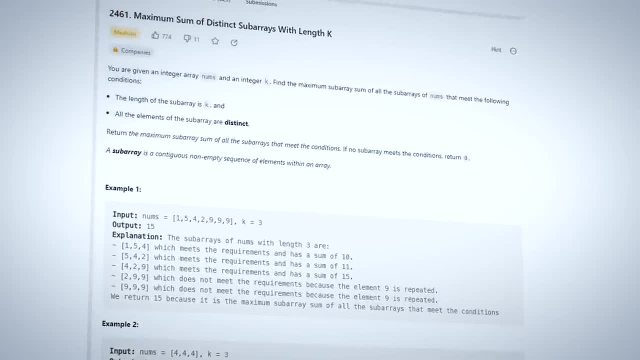 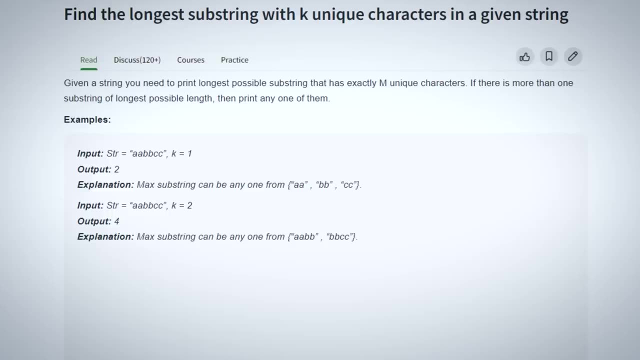 largest substring without repeating characters: maximum sum. subarray of size K and largest substring with K distinct characters. Here we will learn the sliding window algorithm using the largest substring without repeating characters problem. In this problem you are given a string and you need to return the largest substring such that 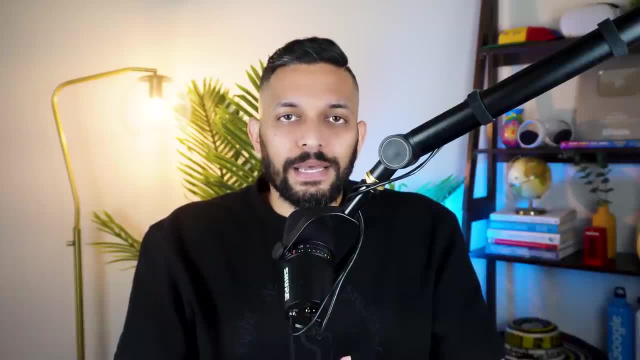 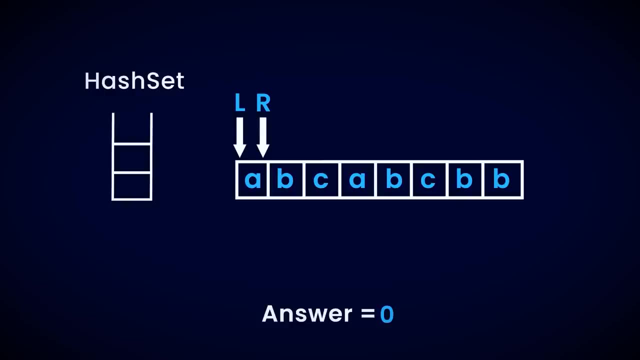 all the characters in it are unique. You can pause the video if you need some time to understand the problem better. In the first step we initialize two pointers left and right at the beginning of the array. Now we increment the right pointer to expand. 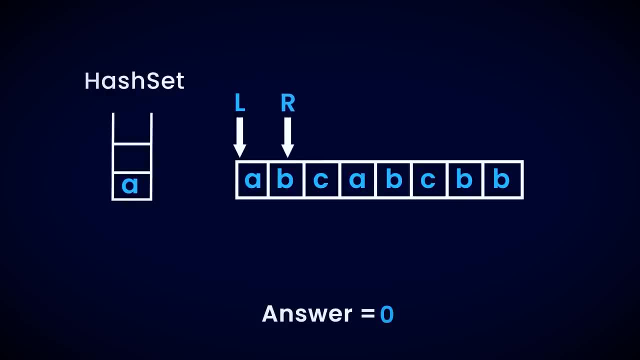 the window between left and right. As we do this, we store the information of all the characters present inside the window. We keep incrementing the right pointer and updating this information until we find a character that is already present in the window. We have reached the 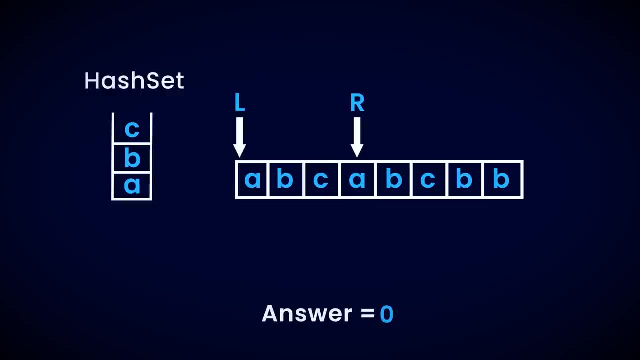 maximum window size because the right index cannot be part of this window due to the repeating character. So we will update the answer here. Now we start shrinking the window by incrementing the left character until the repeating character goes outside the window As we increment the left. 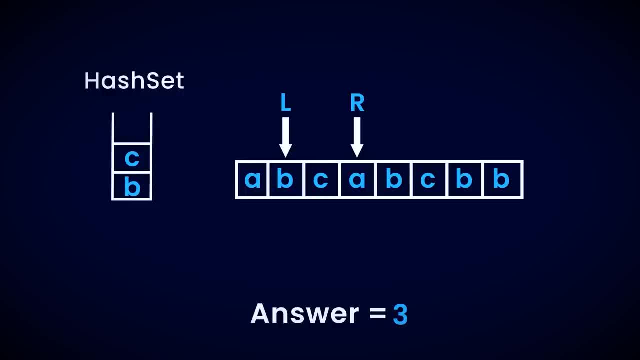 pointer, we will remove the characters that are no longer part of the window from the stored information. Once the left pointer reaches its final state, we can start incrementing the right pointer again to expand the window and repeat this process. We keep doing this until the right. 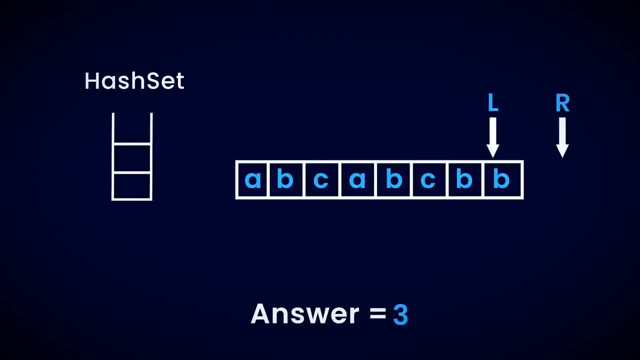 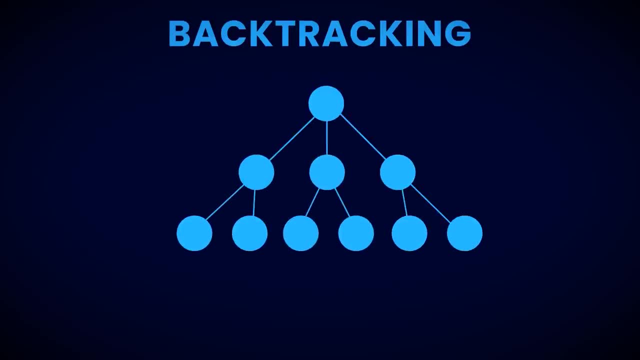 pointer goes outside the range of the array. To help you understand this algorithm better, I will provide a link to the code in the description. At number 3, we have backtracking. In backtracking we explore all possible solutions by building them step by step. When we reach an invalid state, we backtrack or go back. 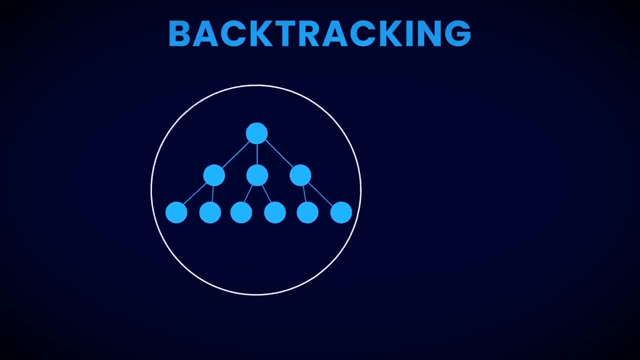 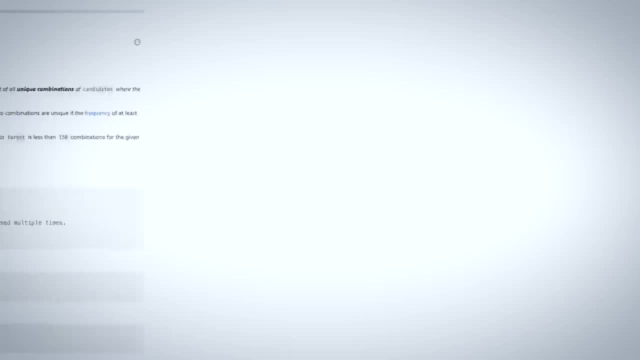 and start exploring the other possible solutions. Backtracking is usually implemented using recursion. I know that none of this makes any sense right now, So let's understand backtracking with the help of a very famous problem called combination sum. In this problem, we are given 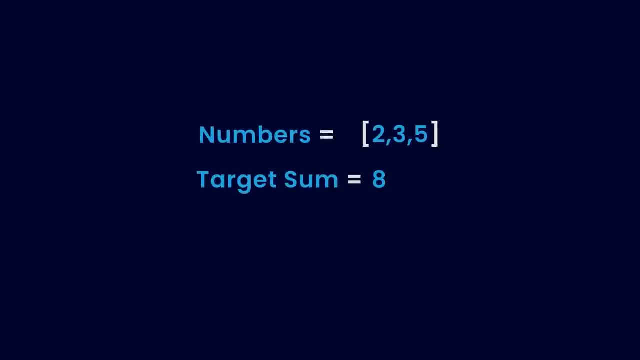 a list of positive numbers and a target sum. You need to pick some numbers from the list so that they add up to the target sum. You need to pick some numbers from the list so that they add up to the target sum. In the end, you have to return all the unique ways or combinations. 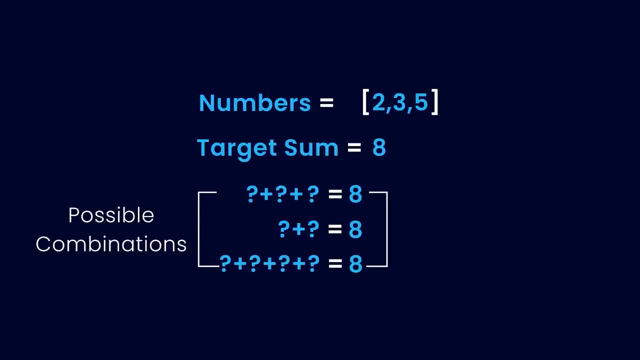 that add up to the target sum. You are allowed to pick a number more than once. In this example, 2,, 3 and 3 add up to the target sum of 8.. So it's one of the combinations in the answer. 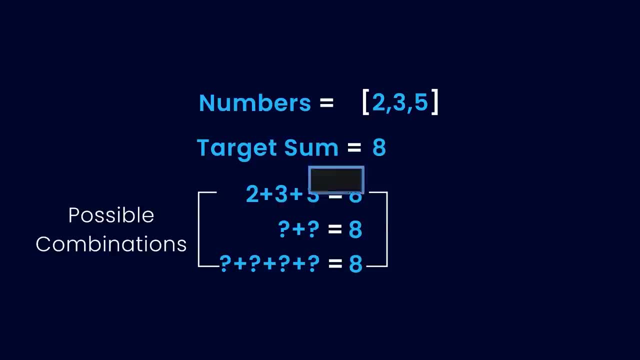 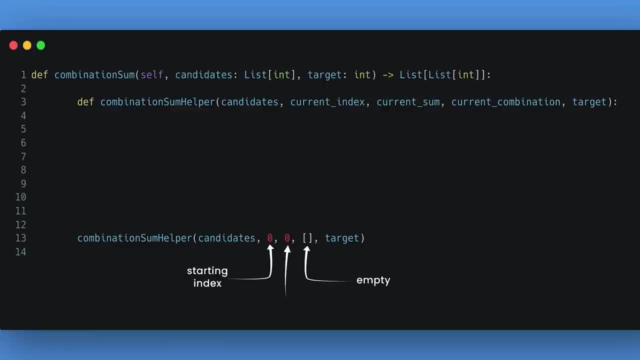 Pause the video if you need some time to understand the problem better. To solve this problem, let's create different combinations from scratch. We start at index 0 with an empty combination and current combination sum of 0.. Whenever the total sum of combination is more than target. 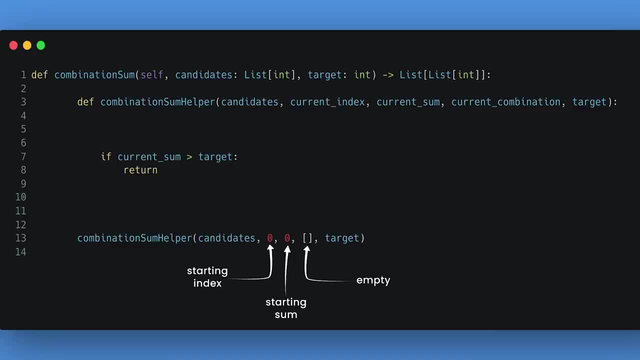 we backtrack or return, because adding more positive numbers to the combination will only increase the combination sum and can't lead to a valid answer. If the combination sum is same as the target, we add the current combination to the answer and return Otherwise for every. 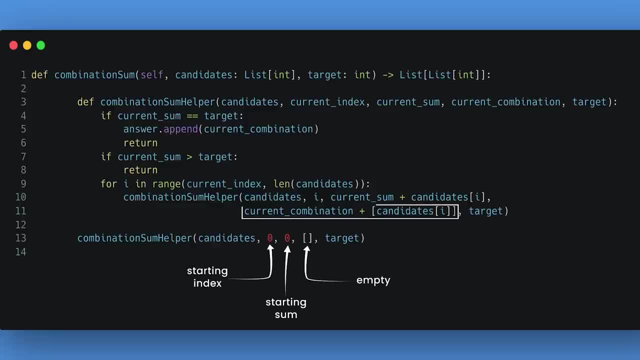 number that comes after current index. we add the number to the combination, update the combination sum, update the current index and call the function recursively. Updating the current index ensures that we only get unique combinations. in the answer I will link the description for you to look at. Backtracking is used in many problems, like word ladder. 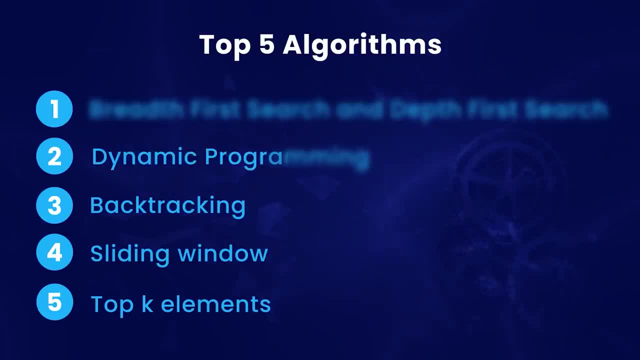 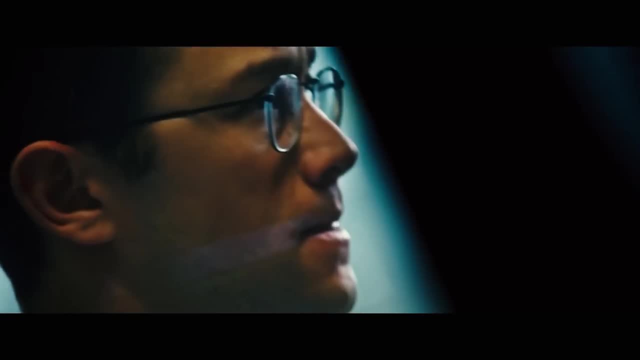 permutations and sudoku solver. At number 2, we have dynamic programming. In backtracking, we explore all possible solutions from scratch, step by step. In dynamic programming, however, we are more thoughtful about the solutions that we explore while still building them from scratch. 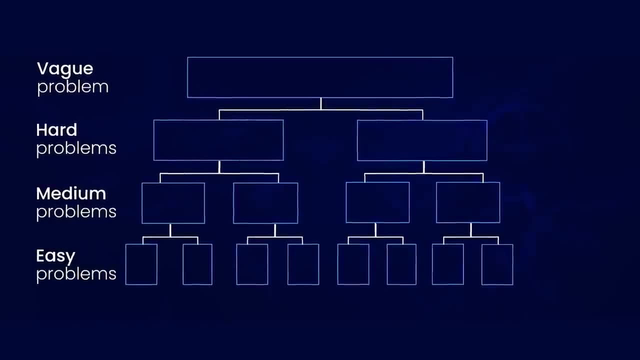 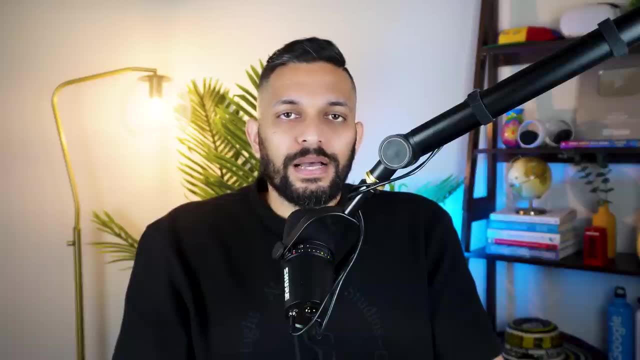 and we do this by breaking the problem into smaller sub-problems. Let's take the example of combination sum again and see how we will solve it with the help of dynamic programming. The problem asks us to find all possible unique combinations that add up to the target sum. 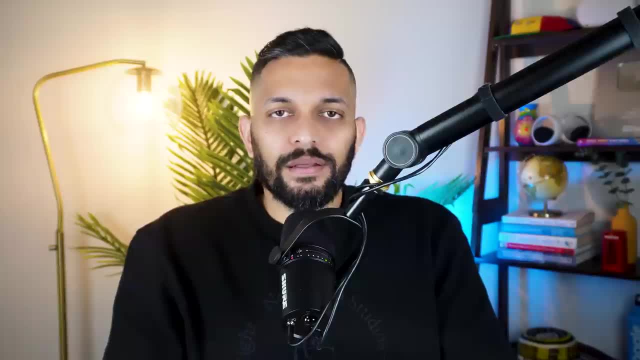 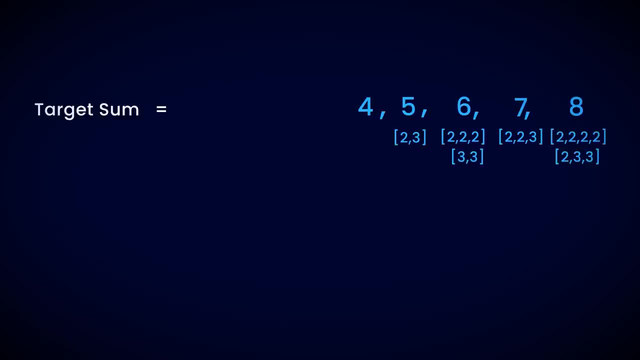 using all the given numbers. But let me change the problem a little bit. Imagine that I give you all the combinations that add up to target sum: target sum minus 1, target sum minus 2, and so on, using all the given numbers except the last one. 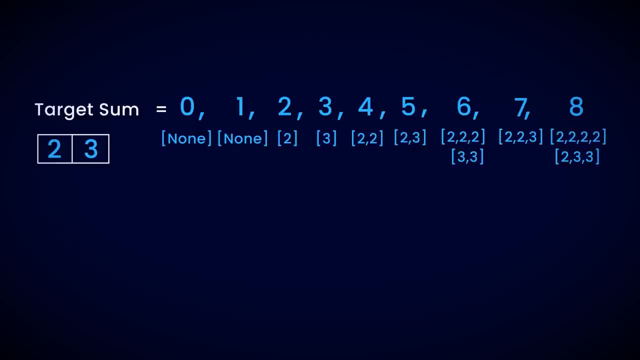 In other words, you know all the unique ways to make numbers from 1 to target using all the given numbers except the last one. And now I give you the last number. Can you use the combination to find all the unique combinations that add up to target, using all the given numbers? 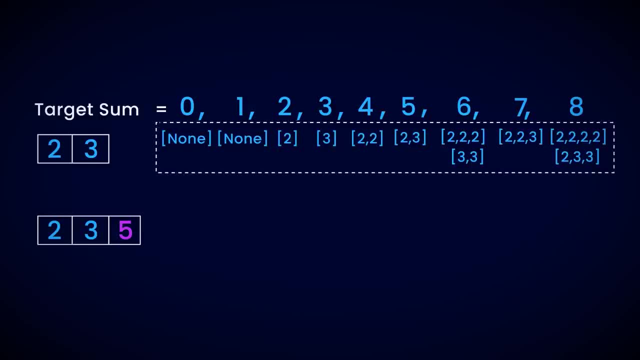 including the last one. You can pause the video and take a moment to think. You can start from the left Until you reach the target sum equal to last number. do nothing For the target sum equal to last number. you can simply add the last number by itself as a new combination. 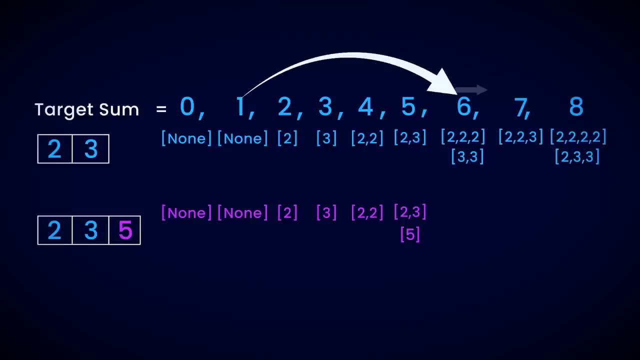 For the target sum equal to last number plus 1, you can just add the last number to all the combinations that add up to 1, and all those combinations would now add up to last number plus 2.. And you can keep doing this until you reach the target sum And voila, you have found your. 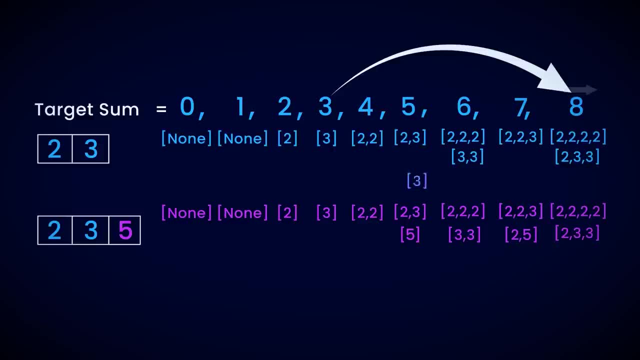 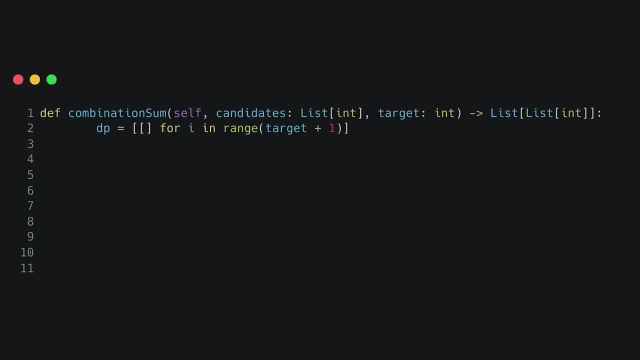 answer. If you look at the code, you can keep track of all the sums from 1 to target using this array. For target sum equal to 0, add a combination which is an empty list. Now start with the first number and keep adding more numbers with this for loop, And for a particular target sum, just add. 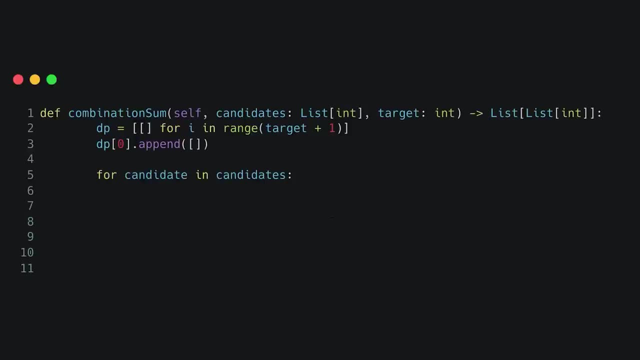 more combinations using all the combinations from the previous list. Now you can add more combinations from the previous list And you can keep doing this until you reach the target sum. For target sum minus current number, I will leave a link to this code in the description. 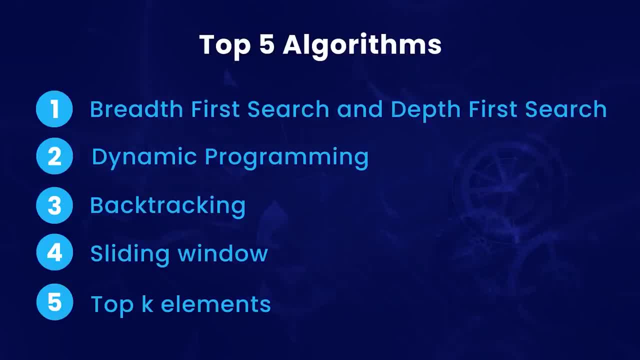 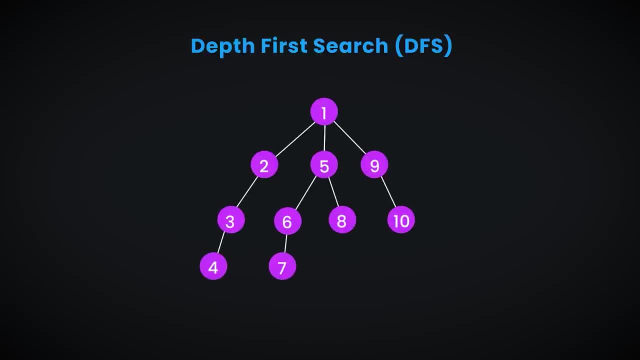 At the very top we have breadth first search and depth first search. I have kept them together because both of them are used for graph traversal and are very similar. Let's start with depth first search, or DFS. In DFS, you start from a vertex and explore as far as possible along each branch. 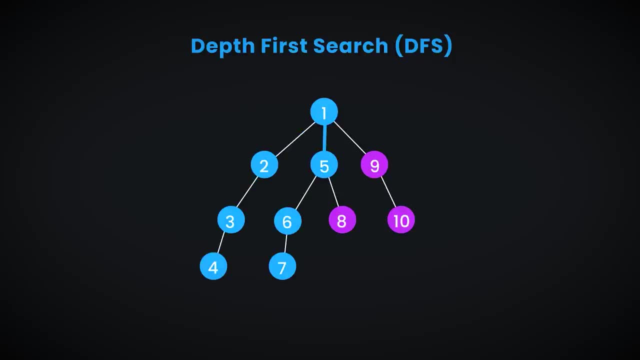 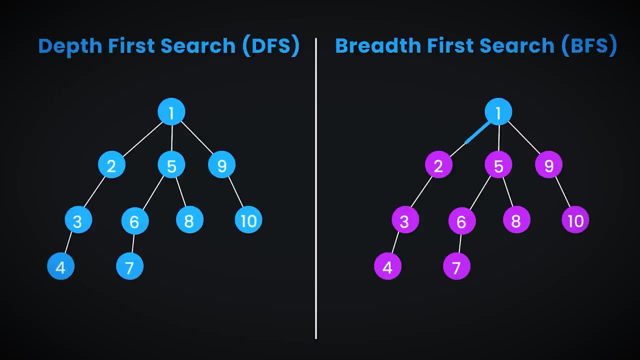 If you reach a point where there is no unvisited neighboring vertex to explore, you backtrack and try to find another branch that is unvisited In breadth first search or BFS. you explore the neighboring vertex first before moving on to the other deeper unvisited vertices. 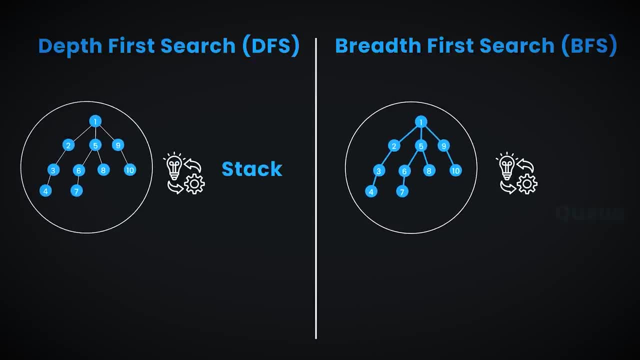 DFS is implemented using a stack, whereas BFS is implemented using a queue. That's because in DFS, you want to explore the neighbors of the last vertex that you visited first, So you want last in, first out, which is what stack does. In BFS, however, you want to explore the neighbors of